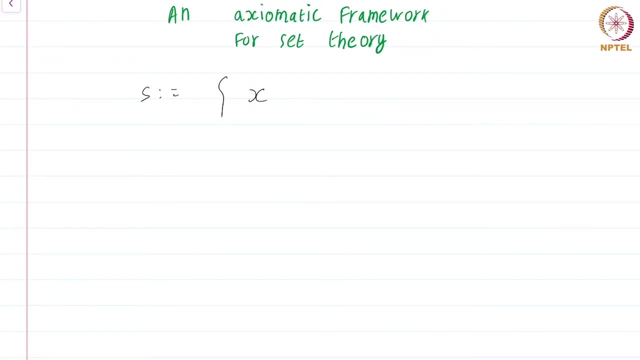 the collection of all elements, such that x is not an element of itself. ok, Just because I have written down a set does not mean that it is indeed a set. Let us see what goes wrong with S. There are only two possibilities. First possibility is that S is an element of S. Well, this cannot. 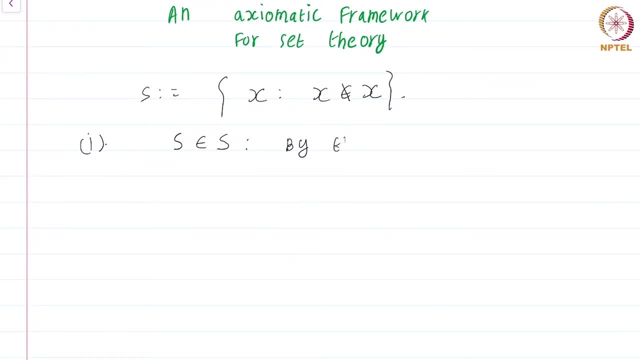 happen simply because, by the very definition, by the very definition, S would not be an element of S. So this is ruled out. The other possibility is: S is not an element of S. Well, then again, by the very definition, S is an S. We end up with a neat little paradox. 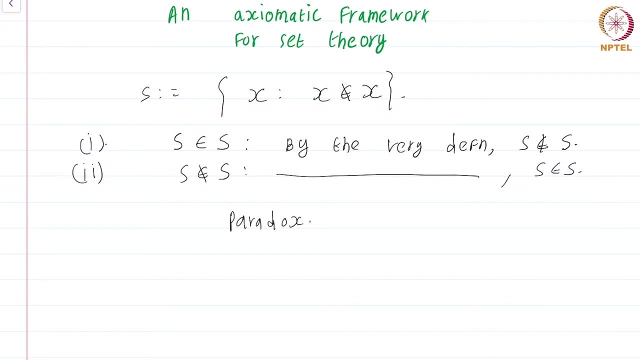 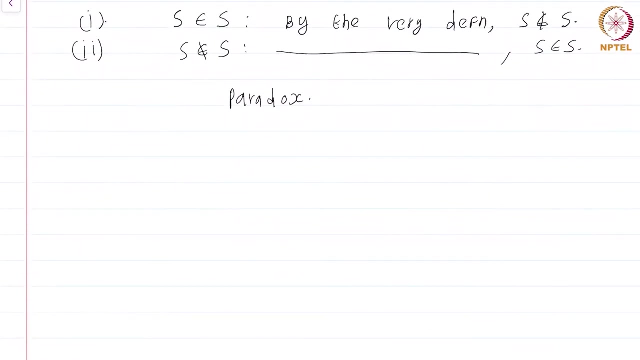 So a paradox is a situation in which both a statement and its negation have some sort of argument supporting them. This paradox shows that if we are not careful about how we define sets we could lead. it could lead up to major issues. There is an amusing version of this paradox. There is a barber who shaves all those and 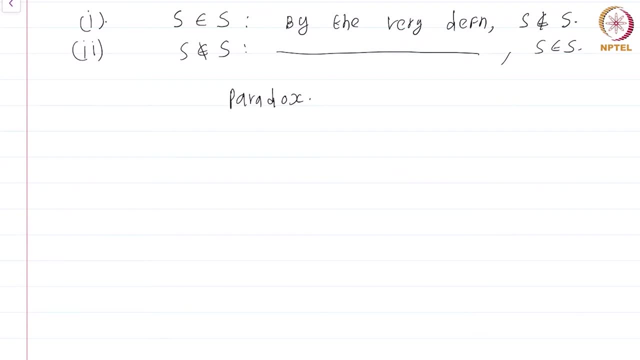 only those who do not shave themselves. The question is: does the barber shave himself? Answering this question results in a contradiction. The barber cannot shave himself, as he only shaves those who do not shave themselves. Thus, if he shaves himself, then he must not. 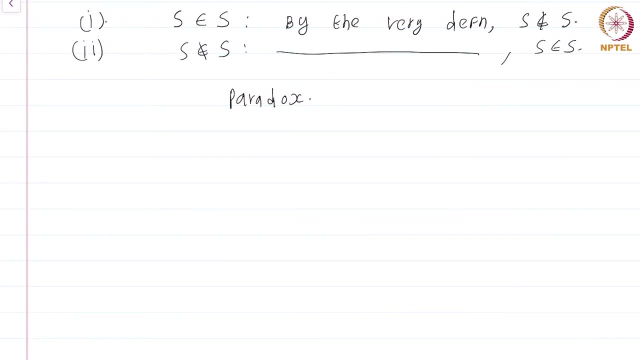 shave himself. On the other hand, if the barber does not shave himself, then he fits into the group of people who would be shaved by the barber, and thus he must shave himself. So this is an amusing version of the paradox, which is somewhat related. 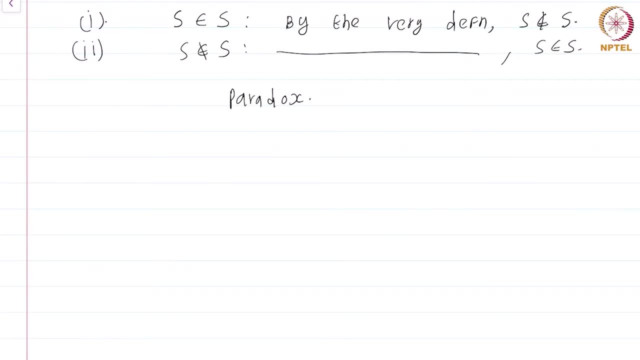 Now the paradox given by Bertrand Russell led to the formulation of modern set theoretic axioms. This was pioneered by Ernst Zermelo in the early 20th century. A bit later, Abraham Frankl and Thorafs Colum independently proposed some modifications. 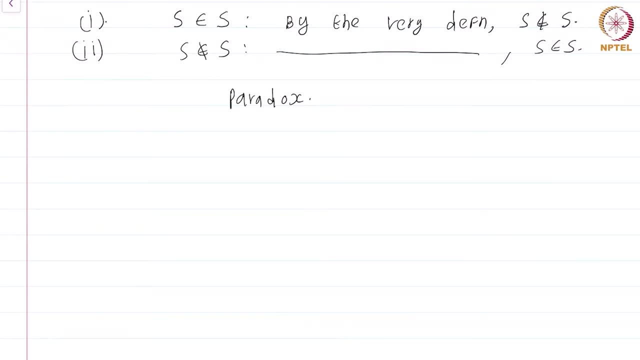 to the axioms of Zermelo, Together with the controversial axiom of choice. this axiom system today is known as ZFC. ZFC acts as a foundation for much of modern mathematics. Virtually every set that you encounter is a set in ZFC. 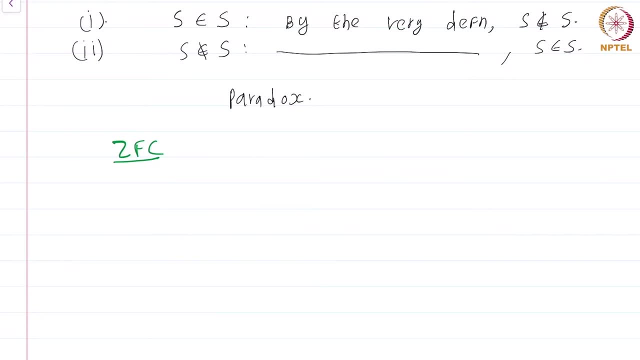 ZFC acts as a foundation for much of modern mathematics. Virtually every set that you encounter is a set in ZFC. There are other formulations of set theory and there are other foundations for mathematics as well, but ZFC is what is used by a vast majority of mathematicians. 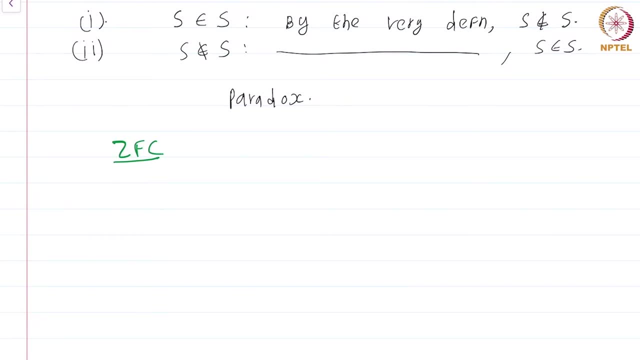 We shall be very brief in our discussion. We will refer to the text of Halmos for more details. In this course, we will not be too worried about set theoretic issues. We will rather concentrate only on naive set theory, which is what we are going to discuss today. 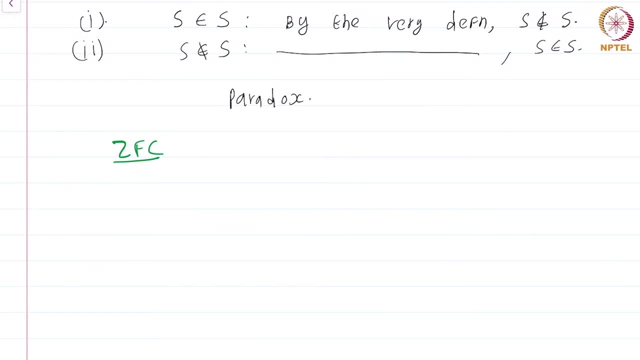 We have seen so far in this course. but it is culturally good to know the axioms of modern set theory, just for cultural purposes. So the undefined terms in this axiomatic framework are: the term set, the relation is an element of, and property. 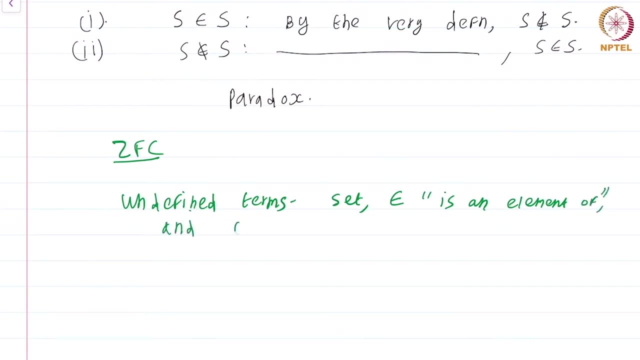 property and the word property. Now, the word property is an undefined term. only in this course, Remember, I just told that Ernst Zermalow's axioms were modified by Thorafs Colum and Abraham Frankel. Their work is primarily to make what this property means more precise. 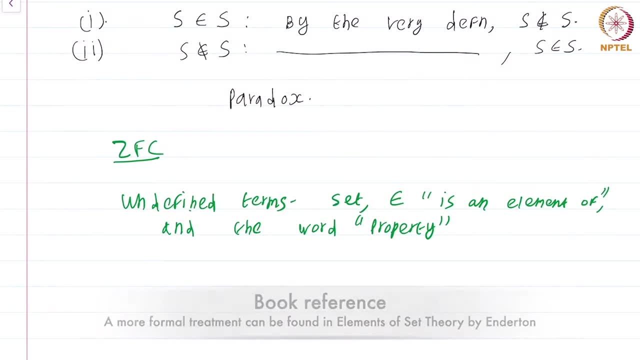 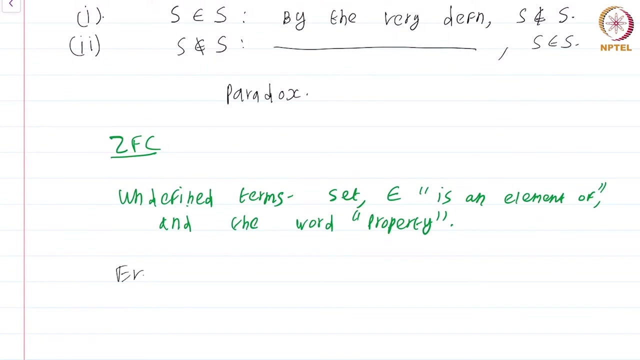 using mathematical logic. So in a course that deals more with mathematical logic, you will see a precise definition of what a property is. With that preliminary said, let us begin with our axiomatic framework. The first remark I want to make is that everything in this 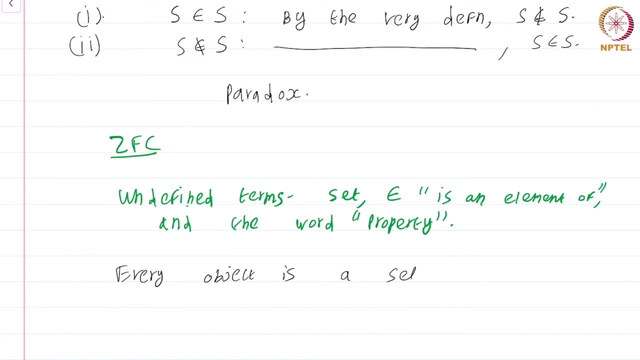 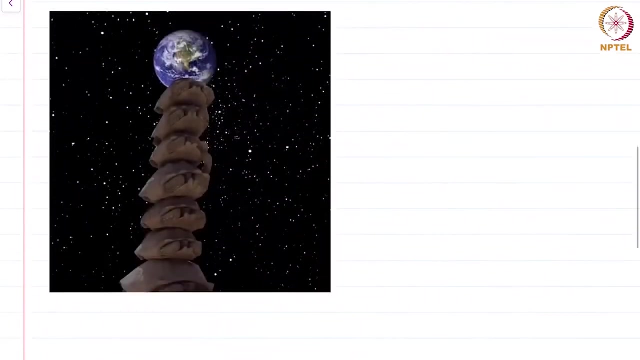 framework is a set, every object is a set. This means that whatever construction which we do, functions, Relations, even more complicated objects like manifolds- which you will see in a future course, no doubt- must all boil down to be sets. In this regard, we have this famous picture of 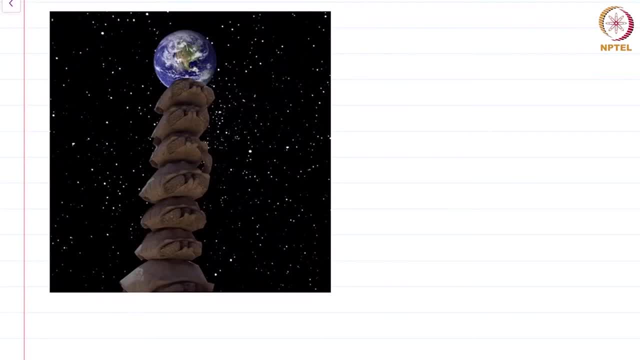 a mythological tale that says that the earth is supported by a turtle, and the question arises: what is this turtle supported on? Well, obviously it is a bigger turtle, and then so on. This is an classical illustration of what is known as infinitesimal. 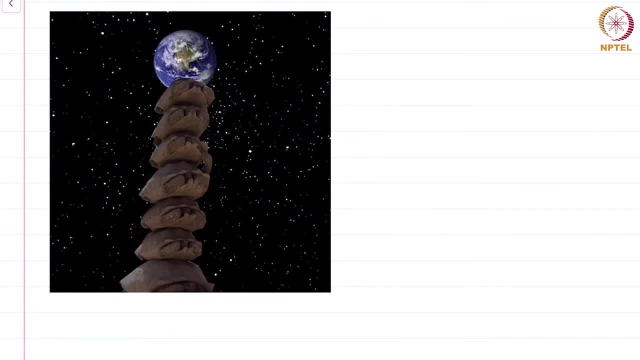 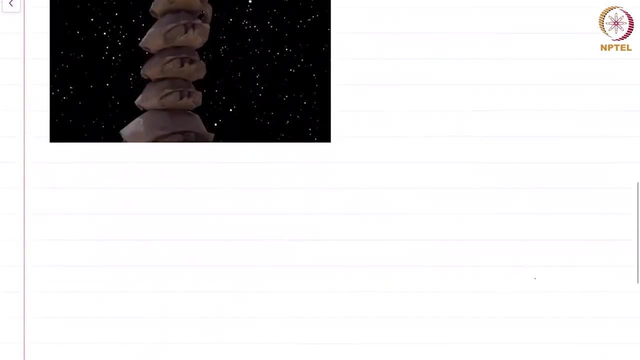 So this is an example of infinite regress. but this issue of infinite regress will not happen in set theory, which we will see in a moment. So we have talked about the undefined terms in this framework. Please remember that they are the term. set is an element of, and. 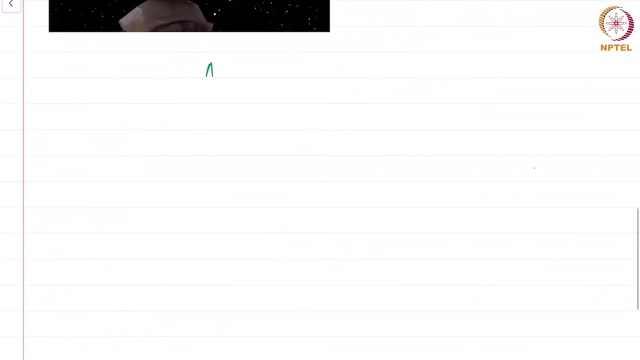 property. Let us list down the axioms. So the axioms of set theory. Now, different forms of sets are different and combinations of sets have different- 快表示- different formulations involved different axioms. What I follow is more or less standard. 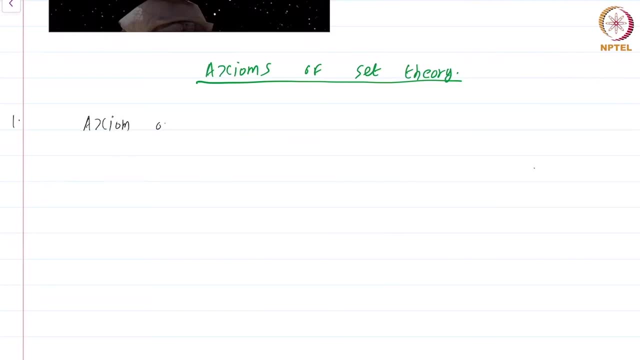 The first axiom is the axiom of extensionality. Extensionality: This says a set is determined today by the spin-off or deflection. Obviously, this is not true for any bigger set. So the axioms are the same in a to ro and si set of set, which I Am, and the machine setup is: 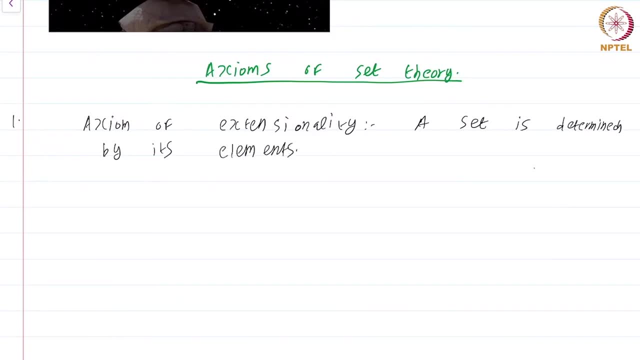 type, but consist by complicating the list What our actual set problem is not question aware by its elements. In other words, two sets, A and B, are identical. Recall in this course. identical always means logically: identical are identical if, and only if, they have exactly. 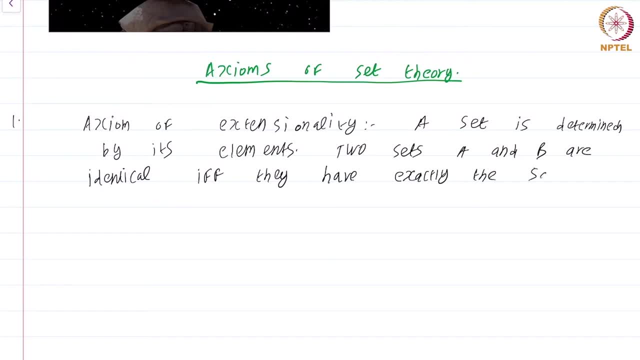 the same elements. they have exactly the same elements. Any framework for a mathematical study should tell you when two objects in that study are logically identical, and this axiom plays that role. A simple corollary of this axiom is the fact that, to show that, 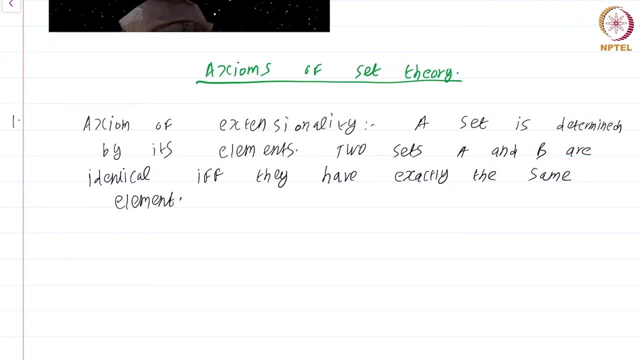 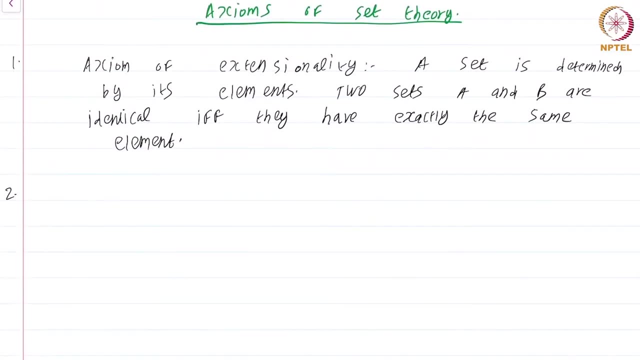 two sets, A and B, are equal. all one has to do is to show that two sets, A and B, are equal. All one has to do is to show that A is subset of B and B is subset of A. The second axiom, which is related to the remark I make about infinite regress not being an 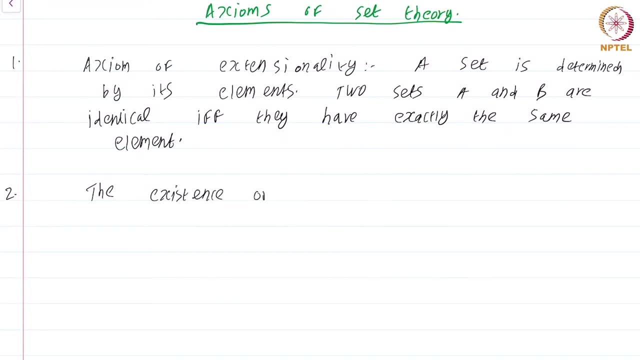 issue in set theory. this is the existence of an empty set. This says there is a set, denoted phi, that has no elements. that has no elements. In other words, if A is a set, A is a set, A is not an element of phi, irrespective of what this A is. Note that I do not use 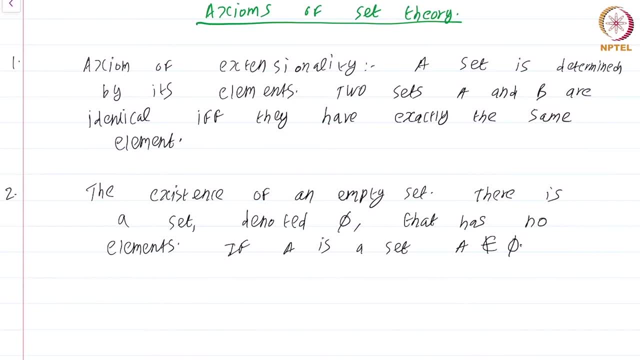 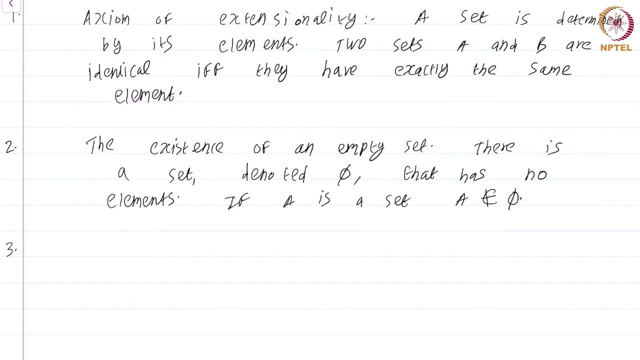 the definite article, the. I say there is a set, there is not a unique set. Well, that is not an issue. I leave it as an exercise to prove that there cannot be two different empty sets. This will follow from the axiom of extensionality. 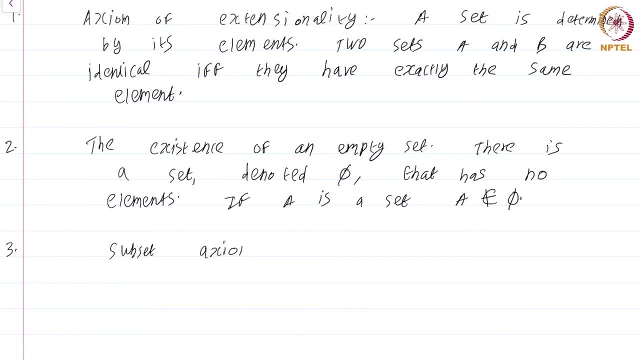 Three subset axiom. This axiom is the most common way to construct subset axioms. The first part is: it is the same C hani. setting a set means if any set will have only two sets order, then of course A is the greater value of B. is it going to be A? But what? 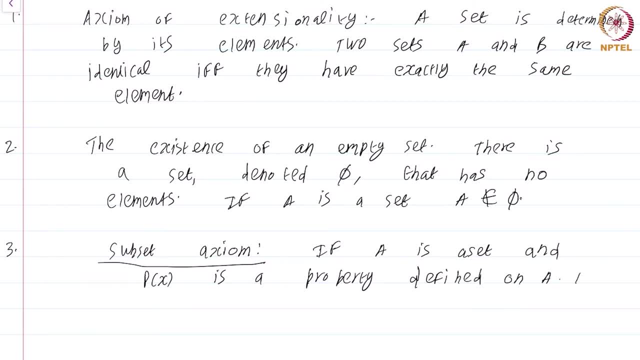 it has to be. Look at C hani. So this I have 52. Joel rices, No C, Really clear. one Fashion table. 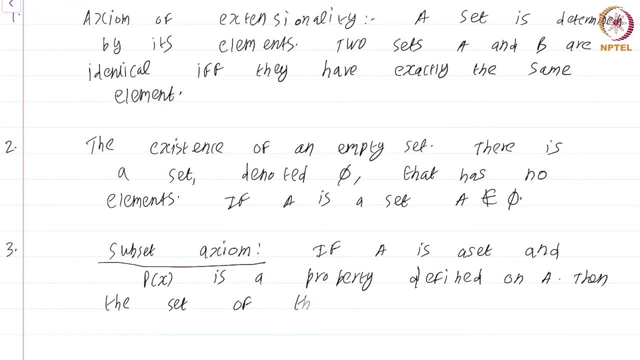 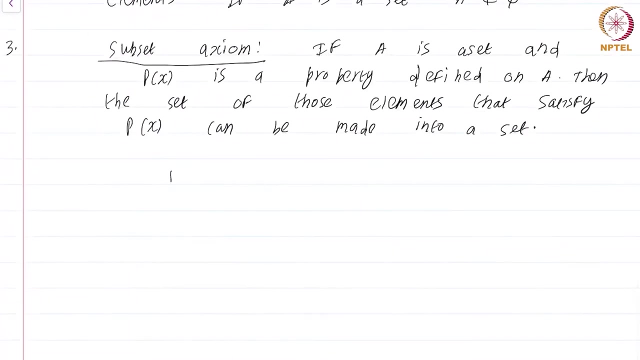 Then the set of those elements, those elements that satisfy P of x, can be made into a set, can be made into a set. In briefer language, if you define B to be x in A, such that P of x is true, then this: 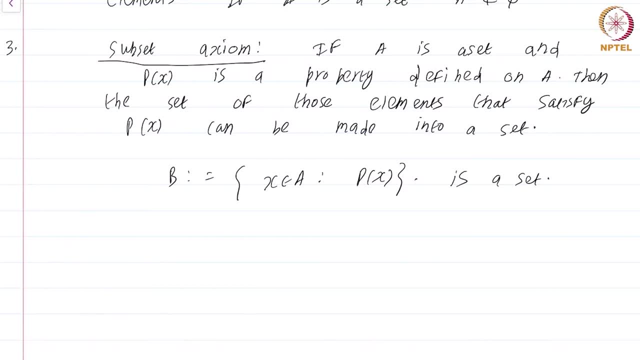 is a set, B is a set. So most sets that we define, we are essentially using the subset axiom and the undefined term property to define them. For instance, the definition of odd numbers, even numbers, prime numbers that we have already. 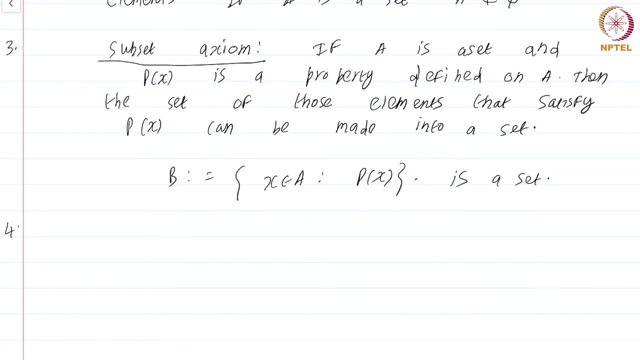 seen. The next axiom is vitally important, especially for this course, because this course, at the end of the day, is about functions. This is the pairing axiom. this is the pairing axiom. This says the following: if A, comma, B are sets, then there is a set of elements that 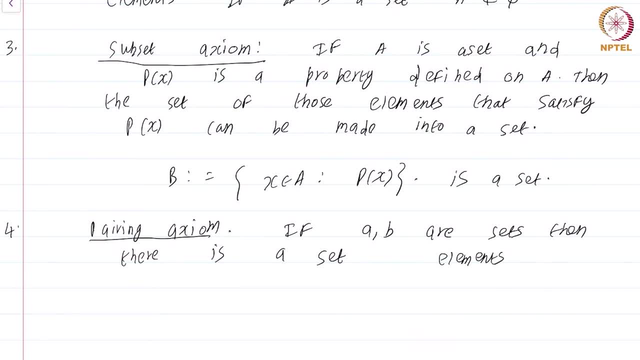 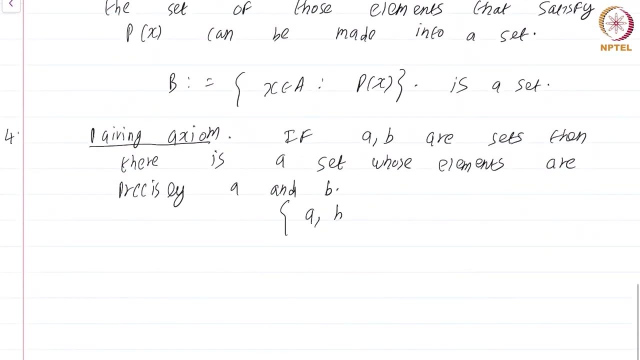 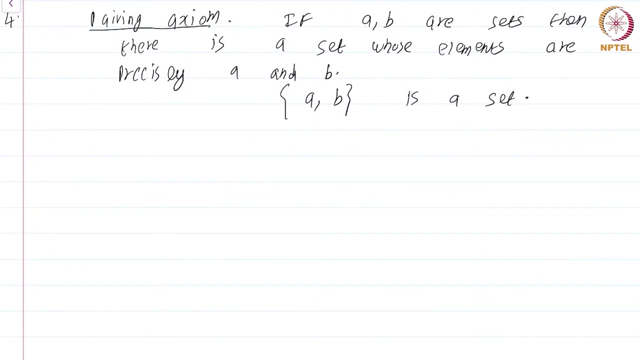 are precisely A and B, rather than saying off elements whose elements, there is a set whose elements are precisely A and B. In other words, A comma, B is a set. Now, why is this so useful? Well, you can use it to construct an ordered pair. you can construct an ordered pair. 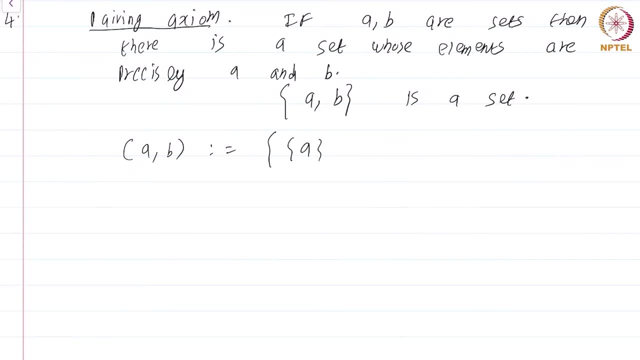 This construction is due to Kuratowski. This. you consider the ordered pair A, comma, B as a set with A and the set with A- B. So it is a set of two elements. The first element is A. I really should not say first element. 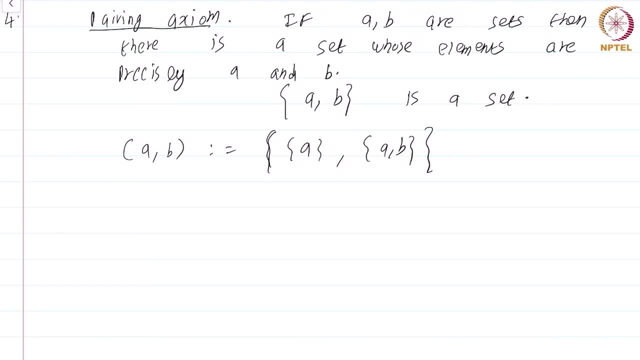 One of the elements is just the set with A and the other element is the set with A comma B. Why does this define the ordered pair? Well, it is an exercise Show that show that A comma B is equal to C comma D if, and only if, A is equal to B. 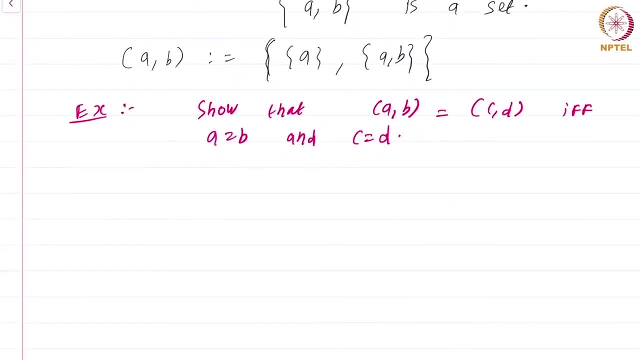 and C is equal to D. Recall from the module on functions and relations that we need ordered pairs to define a relation, in turn to define a function. So this is a set of two elements. So this is a set of two elements. 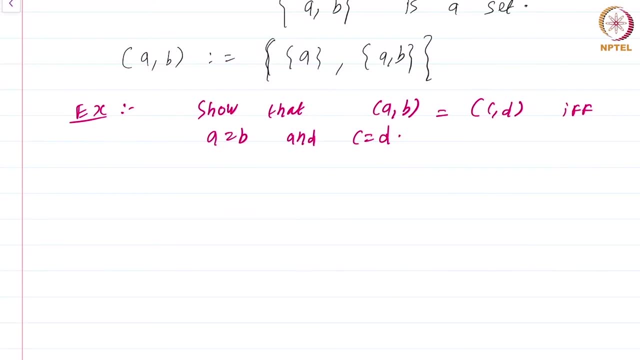 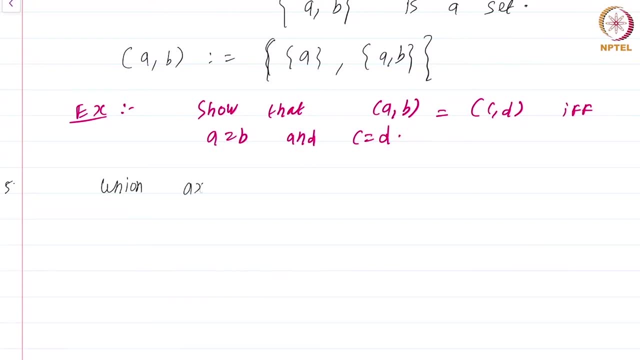 So this is in some sense one of the most important axioms, because this allows us to define functions. The fifth axiom is fairly straightforward: it is the union axiom. It will be stated in a really weird way, because everything for us is a set. 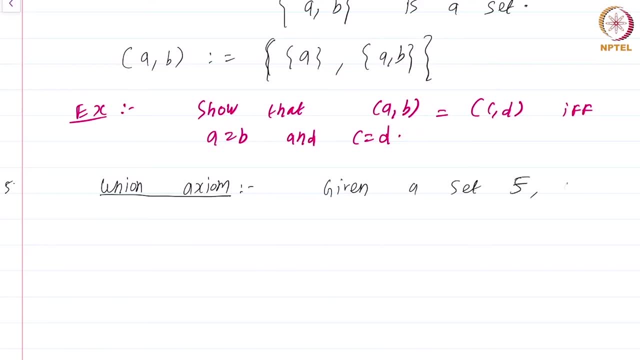 It says the following: Given a set, given a set f, there is a set, capital F. Yes, Yes, capital U, whose elements are precisely, are precisely those that belong to that. belong to at least one element of F. Now recall from our naive discussion of unions: 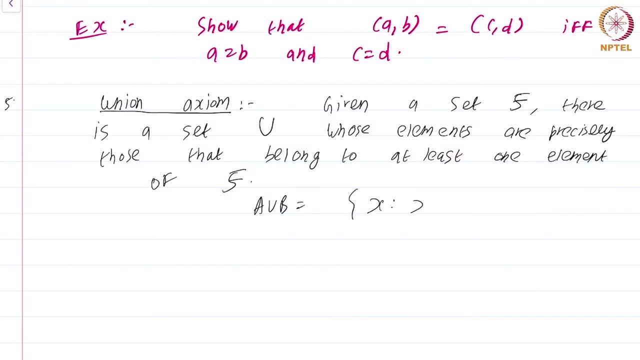 and intersections, that I had defined the union of two sets, A, union B as x, such that x is in A or x is in B, right. But this definition has a problem. It is a problem simply because the property that I am using to define the union it is 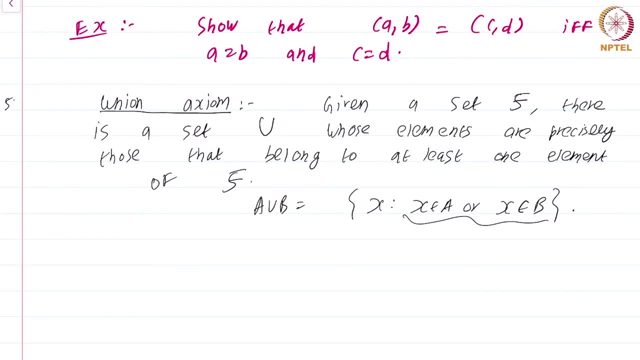 not clear what set it is defined on. Property should always be defined on a set and it is not clear which set this is defined on. This is not really a problem, because the union axiom just says that whatever set you take, you can consider another set whose elements are precisely the elements of the elements. 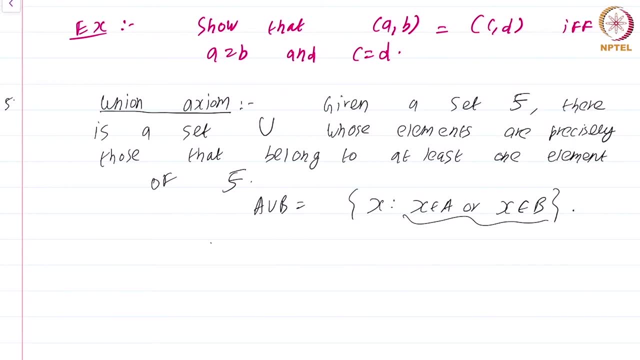 of F, So that is a bit of a word full. So let us, So let me just write that you can. to construct the set A union B, all you have to do is consider the set A comma B, which is a set by the pairing axiom, and then just take the union. 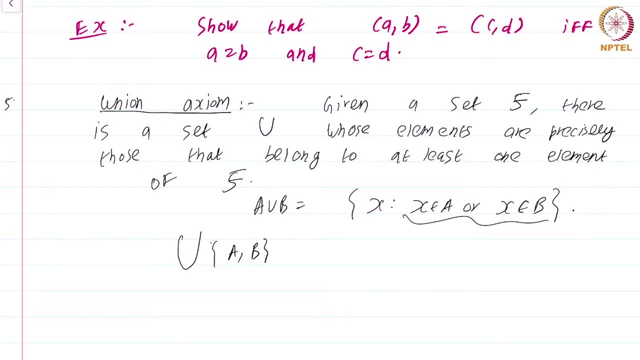 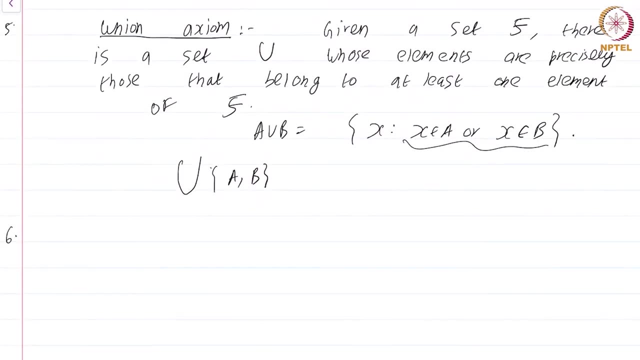 So it is a bit of a convoluted way of just defining the union of two sets. but this axiom is far more general than just the union of two sets. You can take union of any number of sets. 6, the power set axiom. 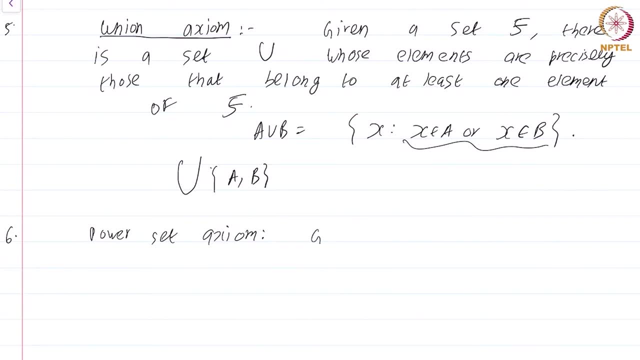 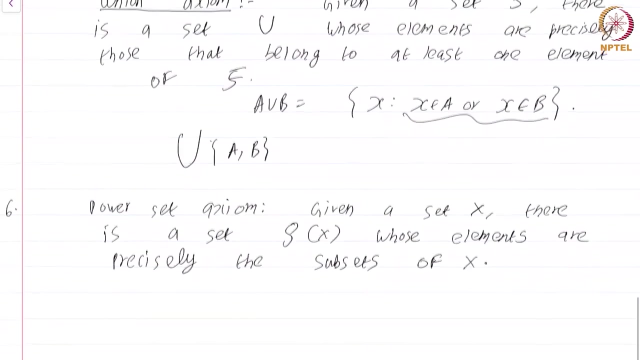 Well, as the name suggests, This axiom is fairly straightforward: Given a set x, given a set x, there is a set. there is a set, the power set of x, whose elements, whose elements are precisely, precisely, the subsets. So this axiom is quite interesting. 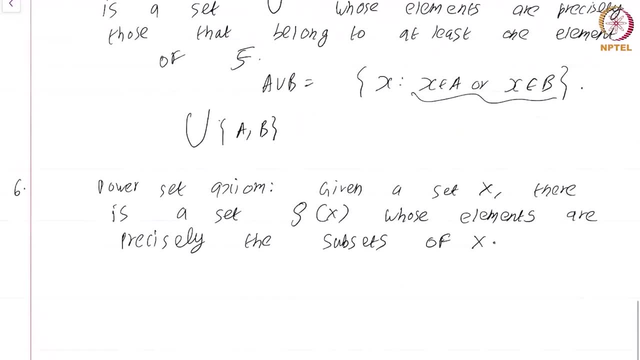 The subset axiom says that, given a set and a property defined on the set, you can extract the subset from that property, but it is not clear whether you can extract every single subset this way. The power set axiom says that, given a set and a property defined on the set, you can. 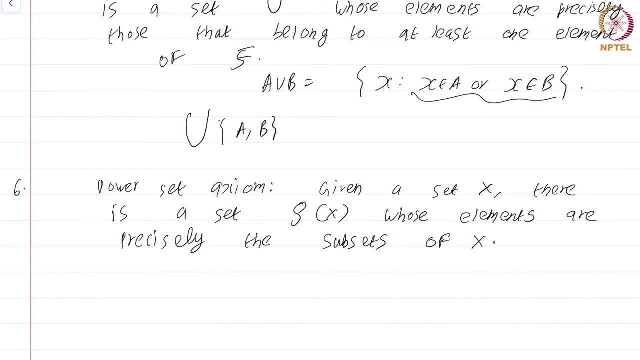 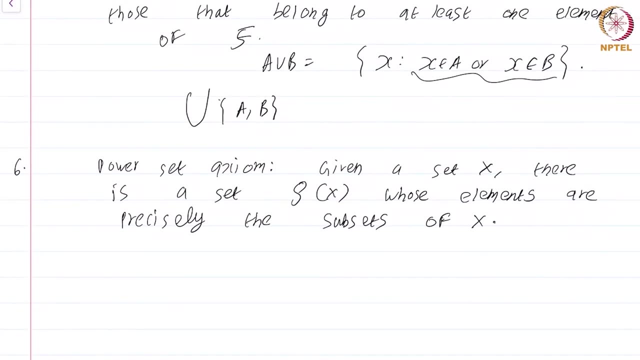 extract every single subset. this way. The power set axiom says that there is a set whose elements are precisely the subsets of x. So, in particular, every subset of x is in fact a set. The next axiom is very subtle. It is the axiom of infinity. axiom of infinity. 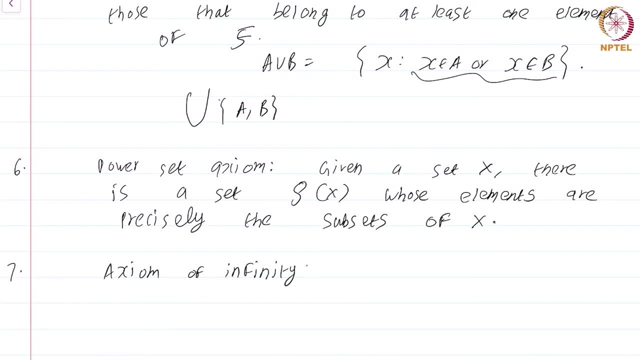 Now. it is a good idea now to pause the video. Look through the first six axioms To conclude that there is no way to produce an infinite set just using these six axioms. If you consider only these six axioms, the only sets that will exist are finite sets. 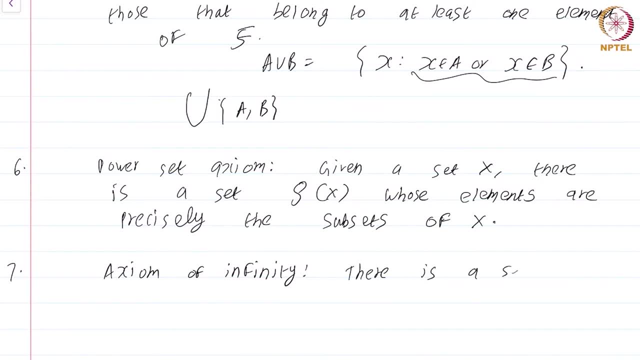 The axiom of infinity says there is a set i that contains- contains the empty set i. So I have taken this axiom. I am going to have an infinity set So we can go to the next slide. Let us see what happens. 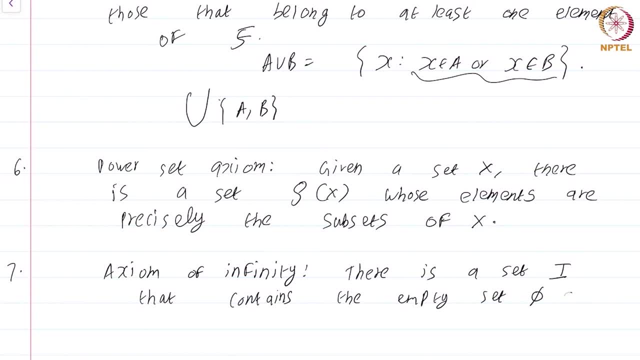 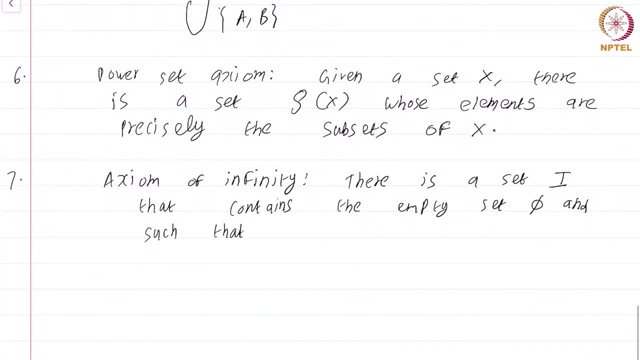 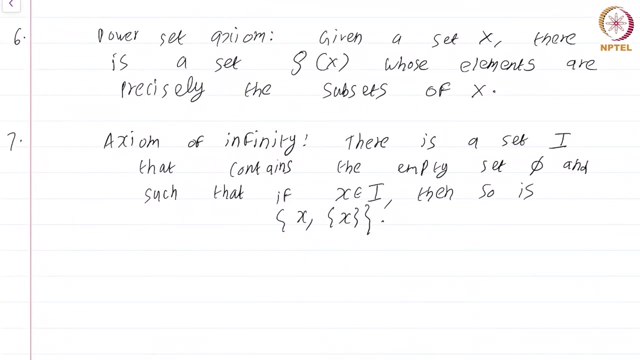 So let us see what happens. phi and such that if x is an element of I, then so is this set, x, comma set with x. ok, Now why does this produce an infinite set? Well, again, I leave it as an exercise Show. 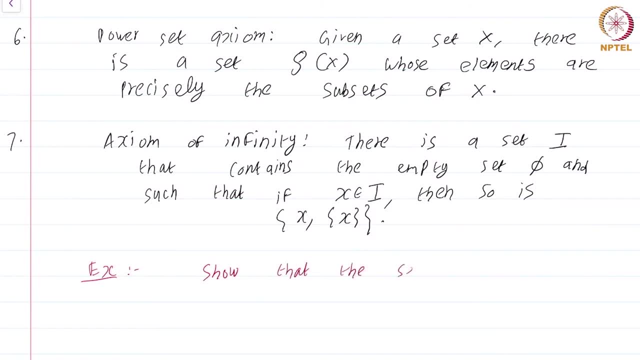 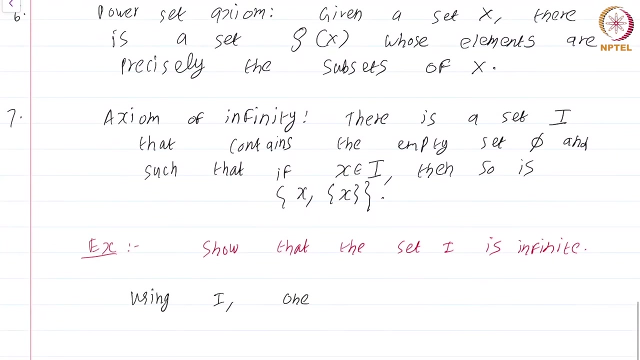 that a set I- is infinite. If you are not familiar with finite and infinite sets, just few modules down the line. we will see cardinality Solve this exercise after I define rigorously what an infinite set is. So this axiom guarantees that there are infinite sets. In fact, using I, one can construct. 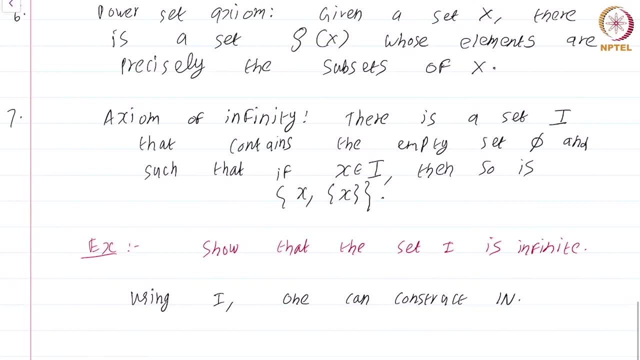 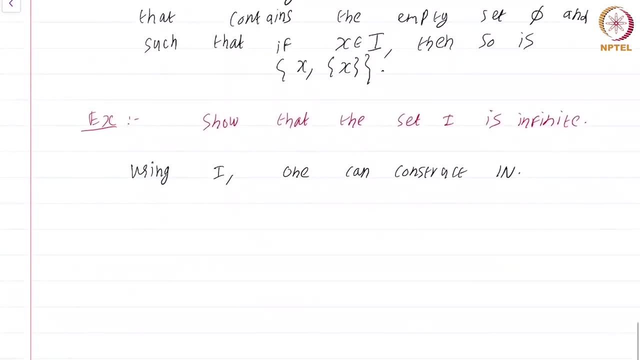 one can construct the natural numbers n. one can construct the natural numbers n, And once you construct the natural numbers n, you can construct all the sets needed in most of mathematics. As a famous quote of Cranucher goes: God created the natural numbers, everything else is the. 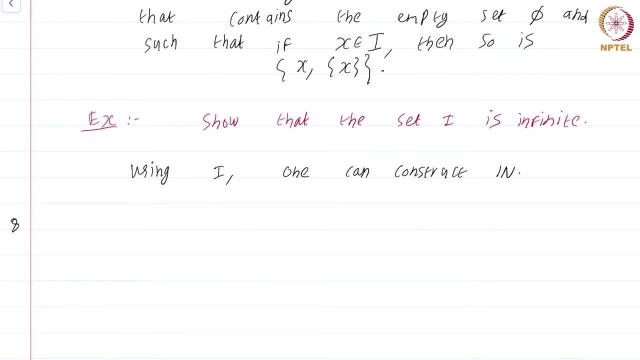 work of man. Now we come to the final few axioms, axiom of replacement. As we go deeper and deeper into this, the axioms become more and more complicated and less and less relevant to this course. This axiom- I am not even sure whether I will ever use this axiom in this. 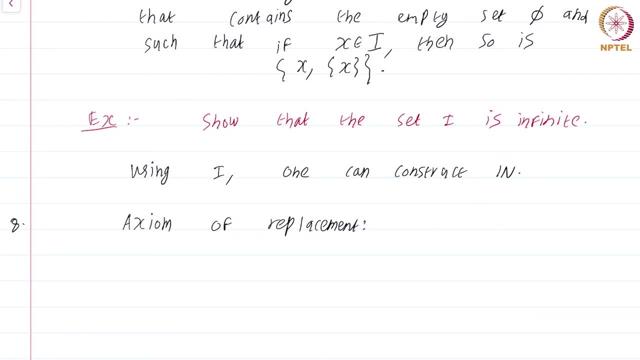 course, but many, many sets I will define and I will be tacitly using them. I will not be using it with my knowledge. So let a be a set and p of x, y be a property, property on a involving two variables involving two variables. Then there is a set B. set B that consists: 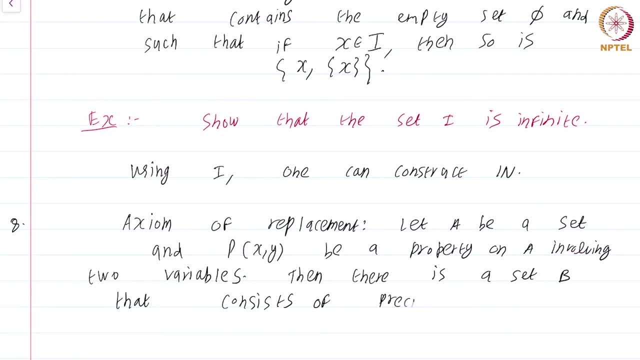 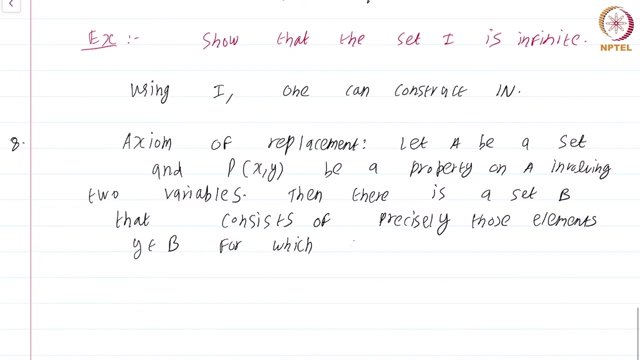 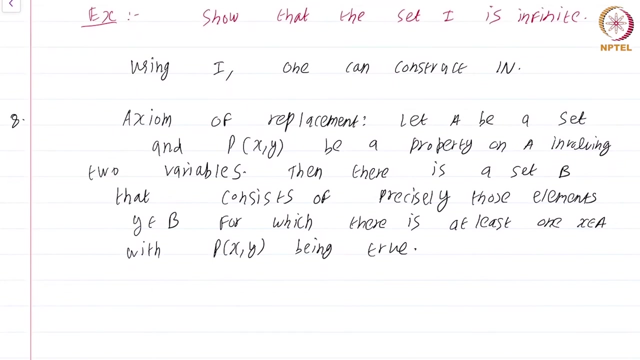 that consists of, precisely of, precisely So, those elements y and b, for which there is, at least there is at least one x in a, with p of xy being true. That is indeed a long sentence and indeed a very, very complicated axiom. This axiom is primarily used to construct many sorts of infinite sets. 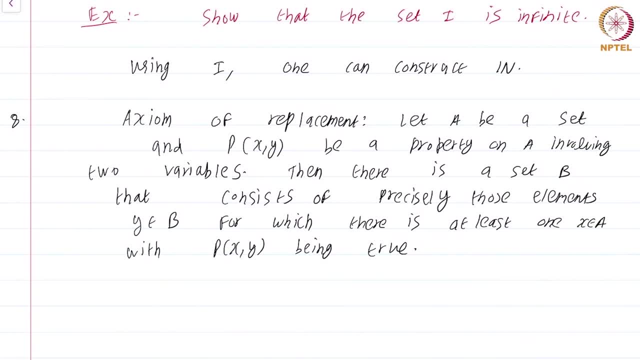 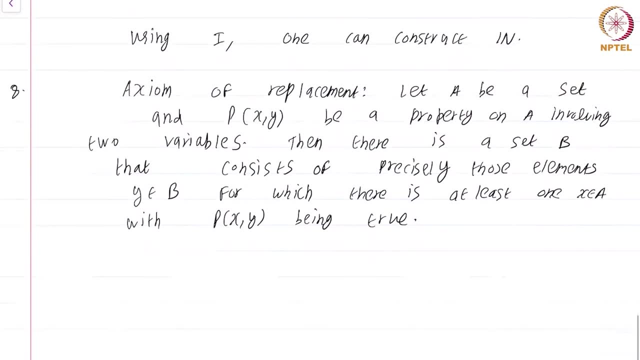 Paul Halmos has interpreted this axiom as saying: anything intelligent one can do with a set yields a set. Now let me explain why this is called the axiom of replacement and in what way we will use it in our course. of course, never explicitly mentioning, never even being conscious, always. 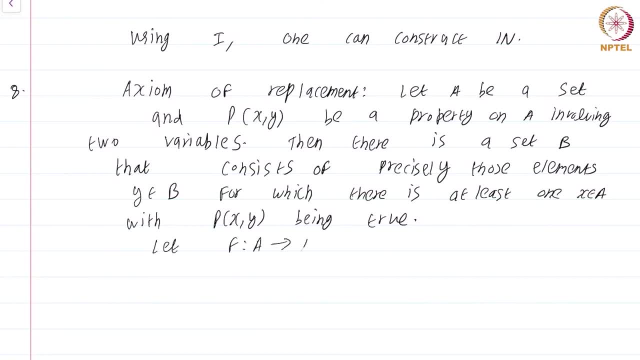 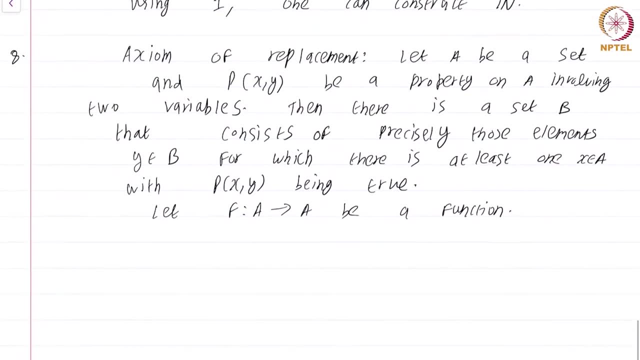 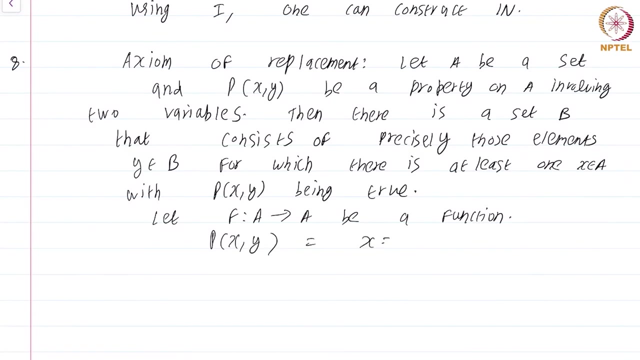 tacitly. Let f from a to a be a function. ok, Then I define the property xy as follows: Property xy is same as saying x equal to f of y, of. sorry, I mean, I had used y and x intentionally to make sure I do not make this mistake. 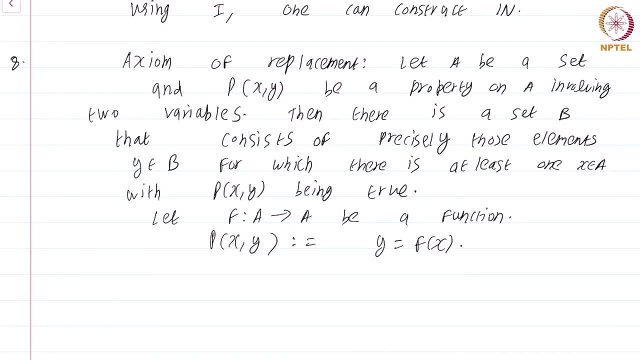 But I still made the mistake. y equal to f of x. Then what this axiom asserts is that f of x, such that x is in a which is exactly same as those elements. y in a, such that p of xy is true. This is a set. 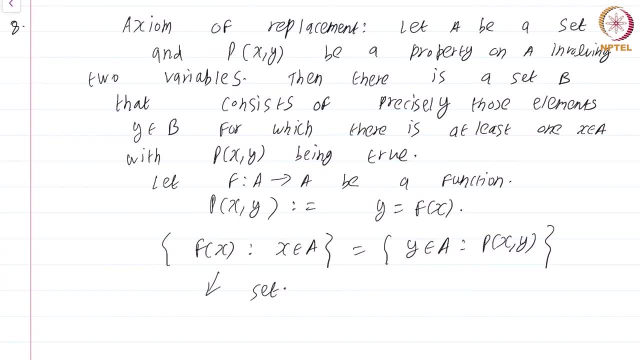 So essentially what I have done is I have replaced the variable x by its image variable y. So in that sense this is called the axiom of replacement. This also says that any function that I can apply to a set will still give me a set that 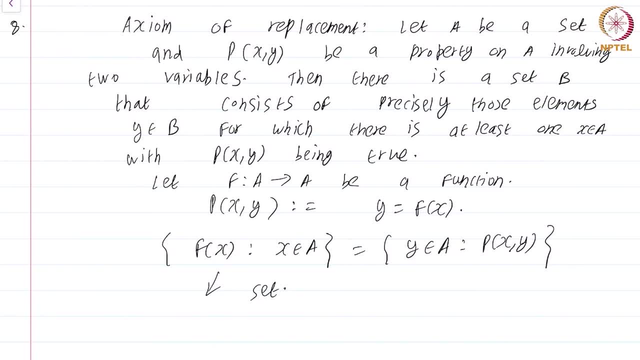 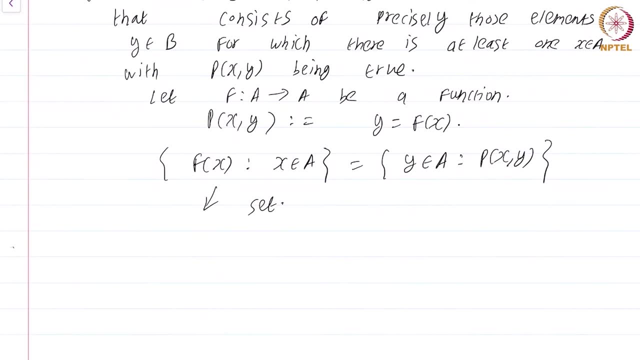 means the image of all functions are sets. So I think now it should be clear what Halmos's quote is trying to say. Now the final two axioms. the axiom of regularity: this is there solely to rule out pathologies Like what we saw with Russell's paradox. 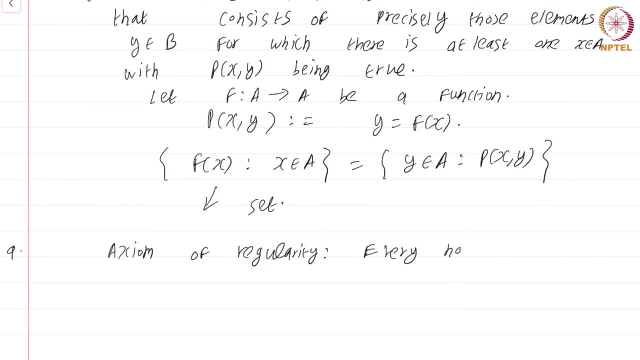 This says: every non-empty set, every non-empty set, a has an element, has an element that is just disjoint from a, disjoint from a. It would be a good idea to pause the video, get some pencil and paper and figure out what this axiom is trying to say. 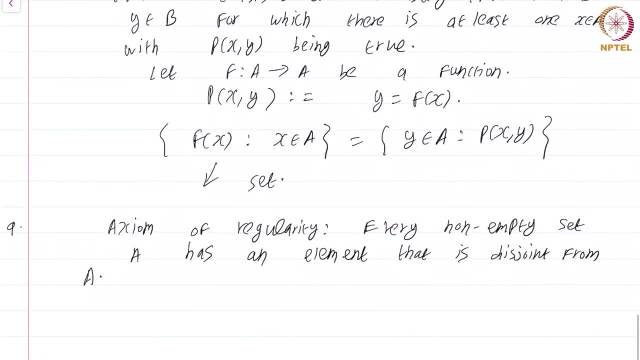 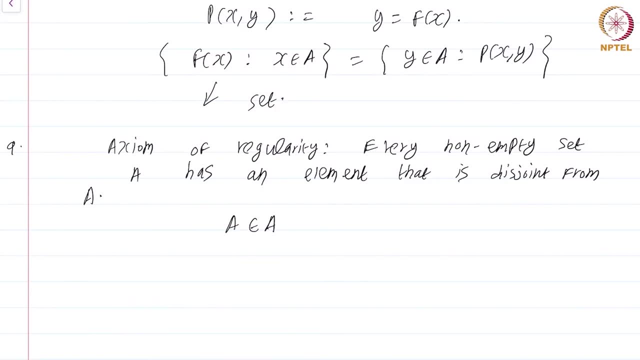 This axiom rules out pathological scenario in which we can have a being an element of a, a set being an element of itself. In fact, you can prove this from the axioms that we have developed. The pairing axiom says: the set with a is a set. 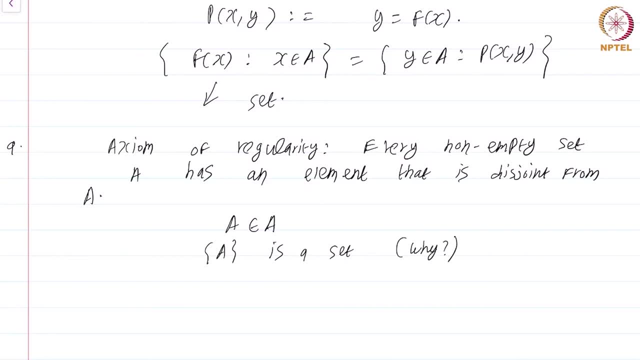 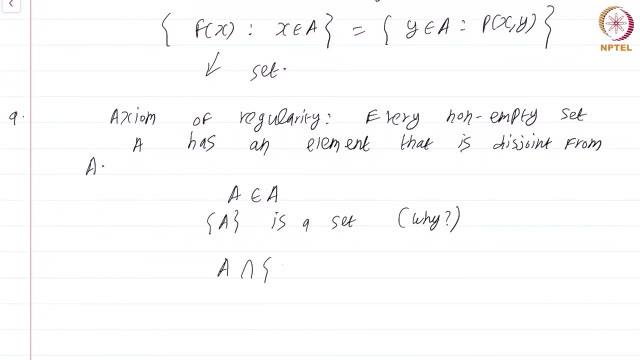 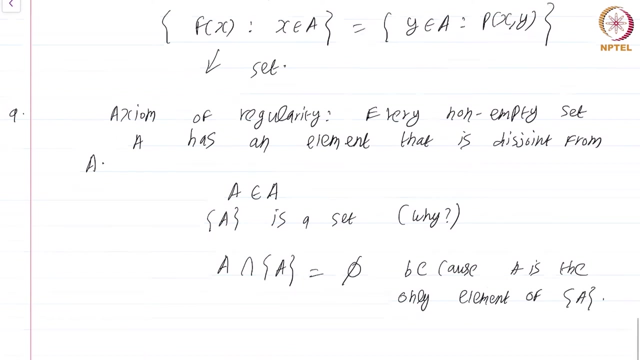 please check why this is true. ok, Now, what does the axiom of regularity say? It says that A intersect set with A has to be empty. Why is this the case? Because A is the only element, is the only element, of set with A. ok, From this, from the fact that A intersects, 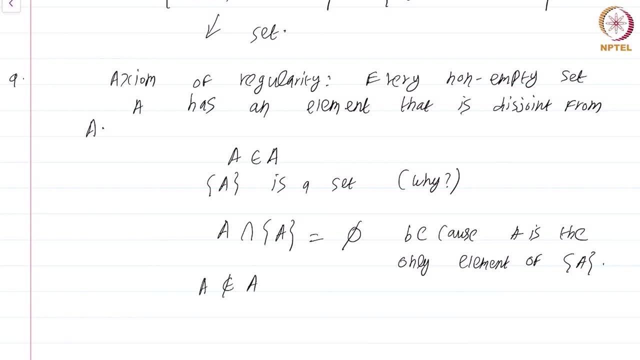 set with A is empty, we can conclude that A is not an element of A. So please pause the video and go through this proof again and make sure you understand what exactly is happening. It may seem like we are just manipulating symbols, and that is true, but that is what. 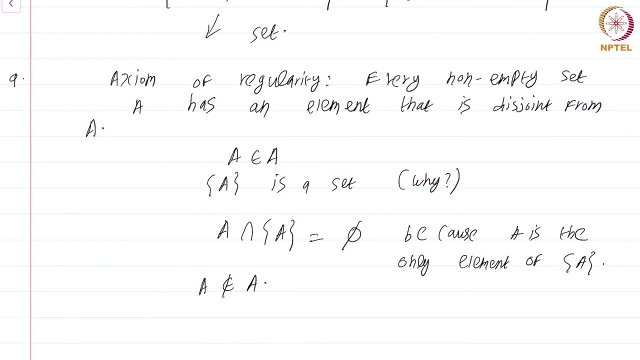 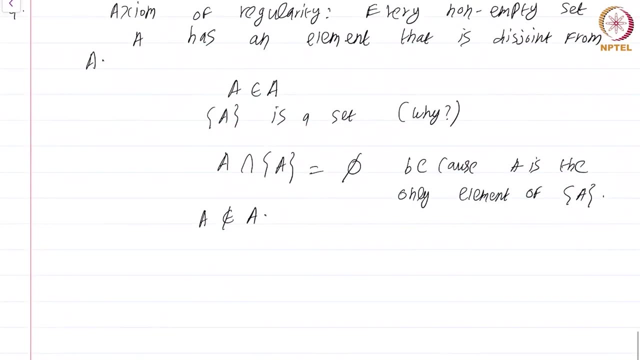 rigorous checking of axioms, rigorous proofs from axioms, actually entails. So this axiom of regularity rules out the paradoxes of Bertrand Russell. And finally, 10, the C in ZFC is the axiom of choice. This is yet another axiom that I do not even know whether I am going. 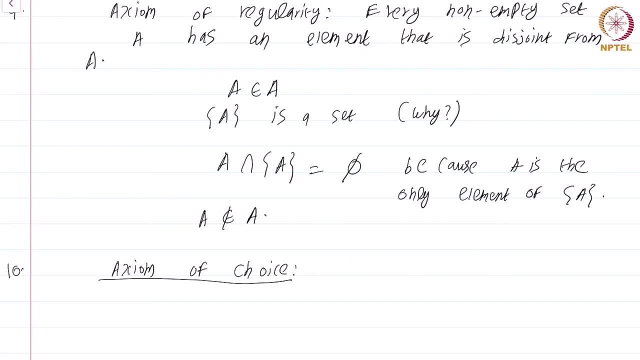 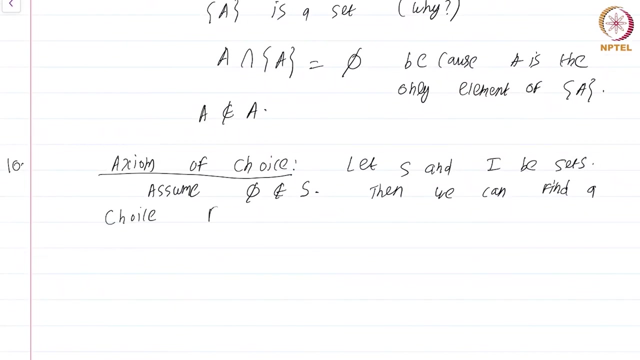 to use. I might use it tacitly without my own knowledge. Let S and I be sets. Assume the empty set is not an element of S, Then we can find- we can find a choice for any set, a choice function. we can find a choice function g from. oh, I missed one hypothesis, sorry about. 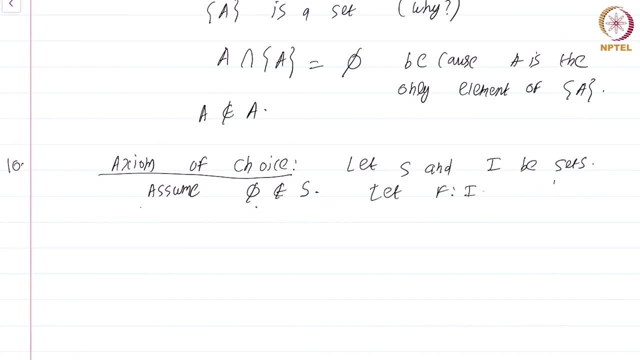 that let f from i to s be a function. Then we can find. find a choice function g from i to s, rather not from i to s, from i to union of s, such that for all i in i, g of i is an element of s. 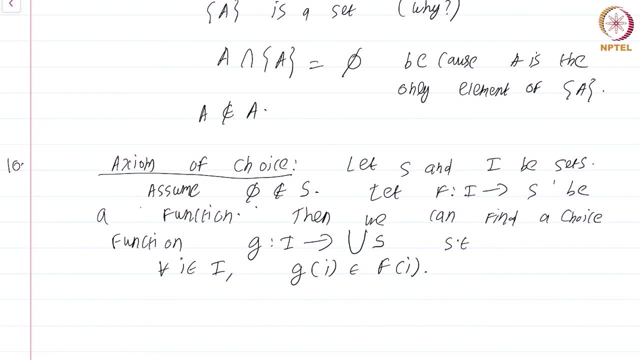 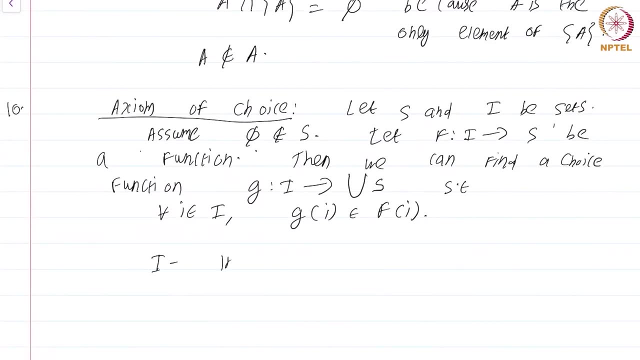 Again a very, very complicated axiom. Let me rephrase what this is saying in plain English. This, i, as you may have guessed, is an indexing set. Essentially, what we have done is we have indexed some sets in the set S. ok, Then what this axiom is saying is that you can find: 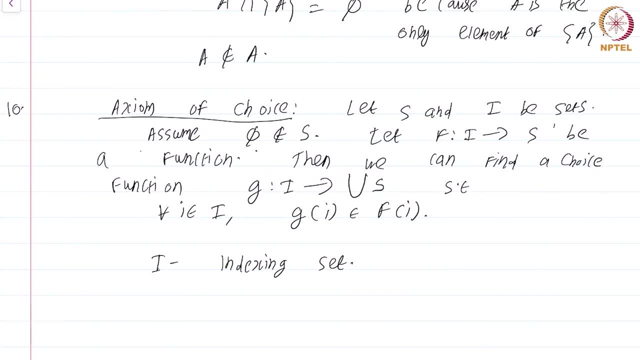 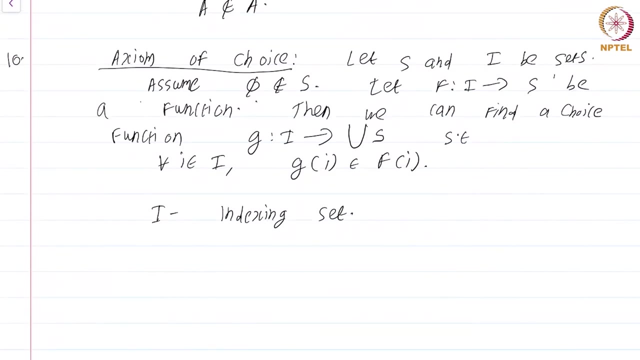 another set Which is precisely one element from each of these index sets. That is what essentially the function g from i to union of s is. It is indexing elements of the elements of s. ok, So this axiom of choice is used in topology extensively. We will only briefly see topology. 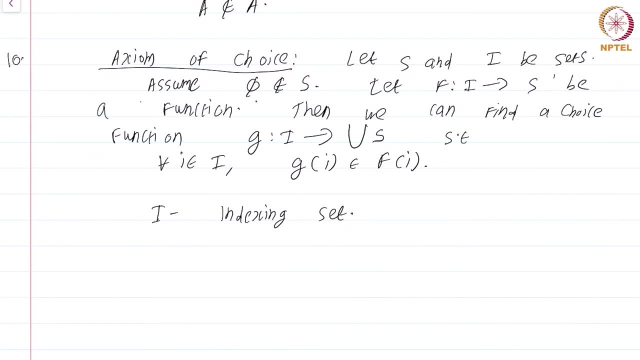 As I say again, I do not really know whether we will use this axiom, but I am sure I will use it without my own knowledge. Let me make some more remarks about this. If the collection S has only finitely many elements, then this axiom is actually not needed. You can produce this choice function by hand. 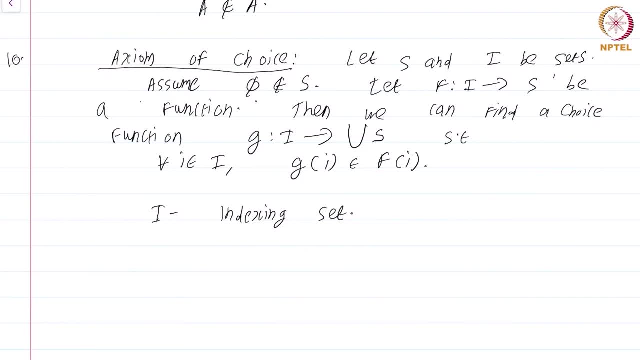 You can use mathematical induction to prove this. There is only one element of S. Then saying that you can choose an element of that set is essentially saying that the set is non-empty. It is equivalent to saying that the set is non-empty, You have to exhibit. 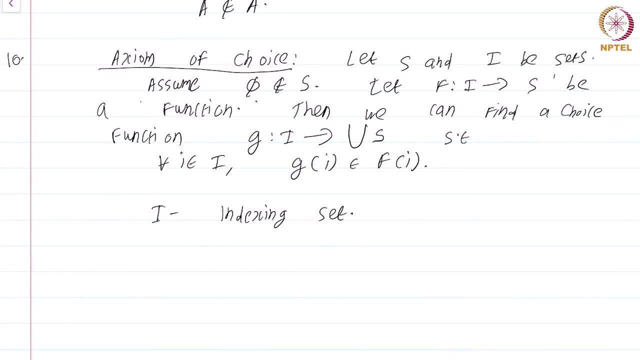 an element to show that the set is non-empty, so that there is no arbitrary choice involved, involved. ok, Not only that, in many other cases also, it will be easy to produce this choice function. For instance, look at the set S. let it be the power set of natural. 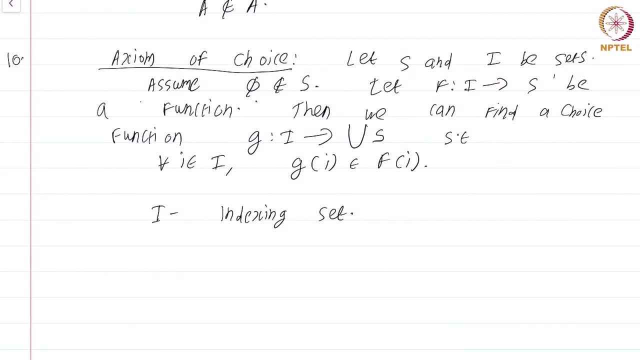 numbers. Later in this chapter on cardinality, you will see that this set is going to be a really vast set. There is no need to inject the set S into the set S. There is no need to inject the set S into the set S. There is no need to inject the set S into the set S into the set S. 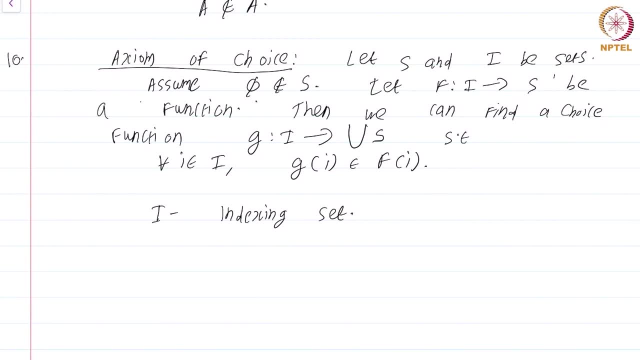 There is no need to inject the set S into the set S. So this is the definition of choice. invoke the axiom of choice to choose one element from each of these sets. Why is that? Well, for each one of the subsets of the natural numbers, there is always a least element. So there is 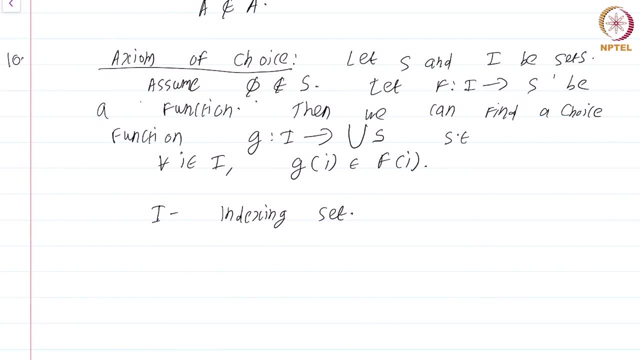 a way to extract the element without using the axiom of choice. So this concludes our presentation of the axiomatic framework of set theory. As I remark again, we will not explicitly cite any of these axioms in this course. In fact, this module is sort of semi-optional. This is just there for. 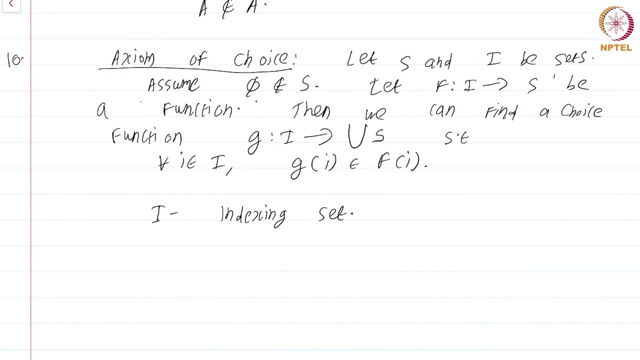 cultural purposes. But let me end by making one somewhat disassuring remark. These axioms we have written down. we have used our intuition and a lot of work on what constitutes the idea of a set. It is clear that the pattern of the set theory is not the same as the pattern of the axiom of choice. 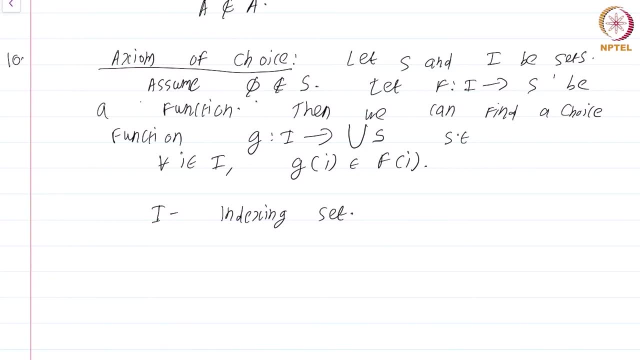 The paradox of Bertrand Russell will go away from these axioms, But it is not clear that there is some other paradox. How you prove that a particular set of axioms never lead to a contradiction is a very difficult topic in mathematical logic. It is so far unknown whether these axioms are all. 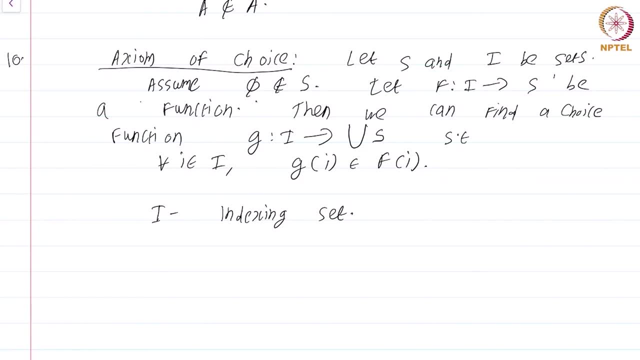 consistent The best result that I am aware of. note: I am not a set theorist. the best I am aware of is that I am not a set theorist. I am not a set theorist. I am not a set infomercial. The practice of a set subject when I work through my fields at higher office is: 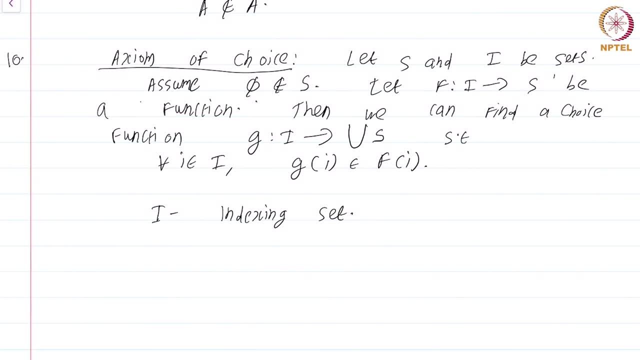 that if the first nine axioms do not lead to a contradiction, then the addition of the axiom of choice will also not lead to a contradiction, even though something is lie. For this reason, we write whether the plus and minus axioms of a set, such as a set, will lead to a contradiction. 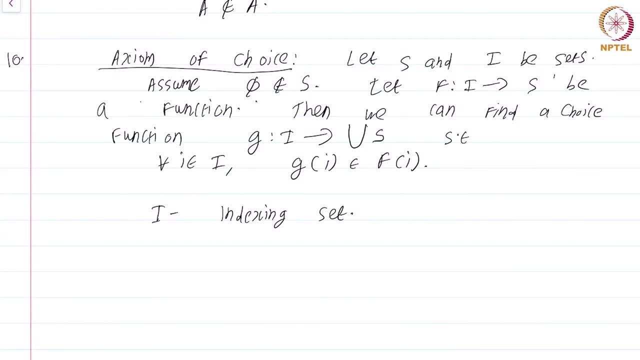 But when something strange happens, even if you add the negation of the axiom of choice, there will still be no contradiction. These are path breaking results of the mathematicians Kohan and Kurt Gödel, So there are a lot of deep issues involved. Since this is: 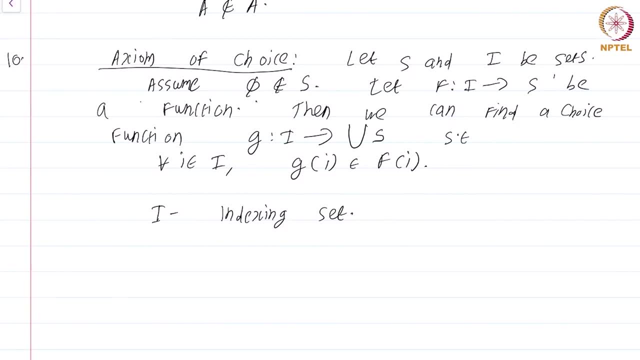 seventh episode: scripture, logic and so forth. I would like to finish off my deck. The answer for this question is as follows. we are going to spend minutes reading the first course on analysis. this itself is a bit too much. So if this particular module 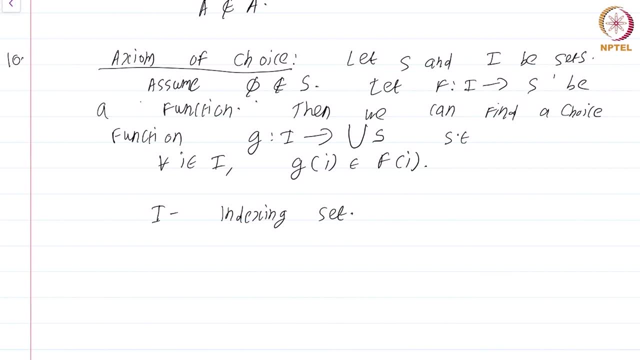 is a bit difficult for you, do not worry. this is just there for anticipating the future. If you are really your interest is peaked by this module. please read the book of Halmos. it is an excellent book. This is the course on real analysis, and you have just watched.